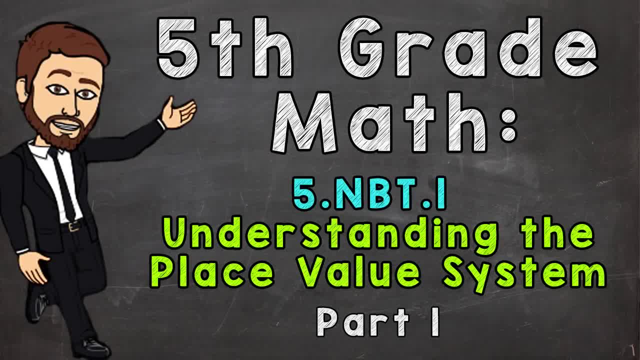 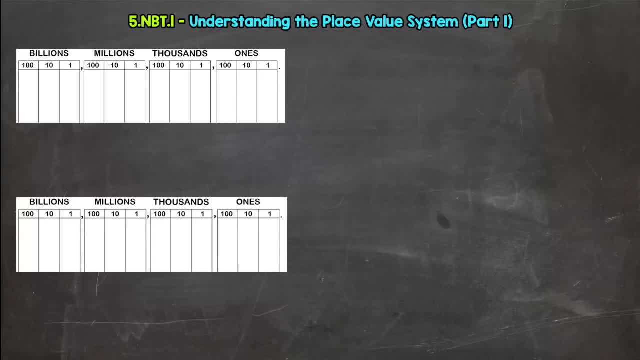 Welcome to 5th Grade Math with Mr J. In this video we're going to be talking about standard MBT.1.. And if you don't know what that means, that's fine. It's basically about understanding the place value system And, as you can see below, I have two place value charts. Okay, 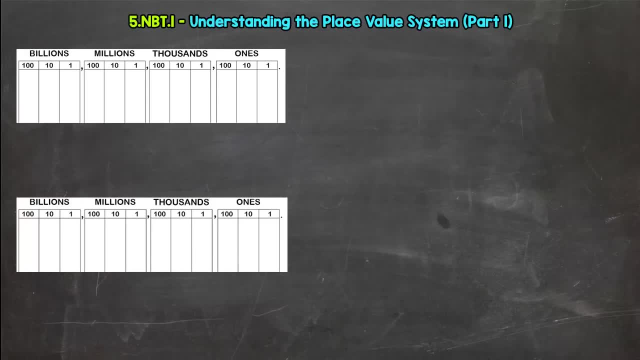 we're going to be working with both those, But let me back up here for one second. This is part 1 of two instructional videos, So there will be a part 1 and a part 2. And then I'll follow part 1 and part 2 up with a mastery check where you can do some on your own to 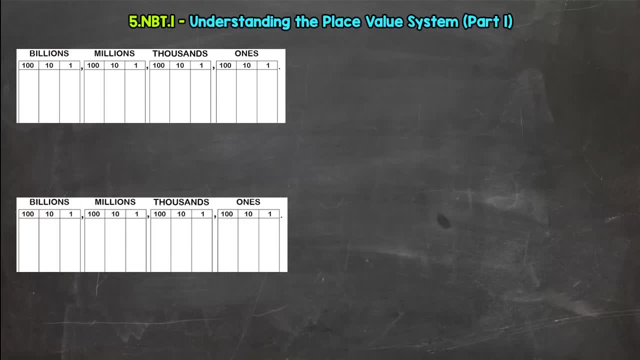 see how well you understand this, And we're going to be talking about relationships between places in the place value system, And I'll show you what I mean here in a second. So let's start with this top place value chart And we're going to start with a 2.. Let's think about the number 2.. If it's in the 1's place, 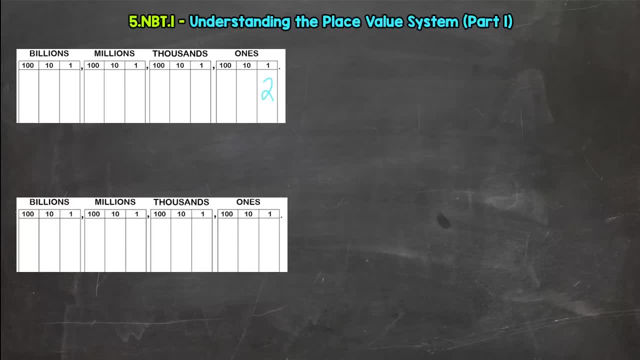 it's worth 2.. Its value is 2.. How about if we push it one place to the left, to the 10's place? Now we have a 20.. So we're going to talk about what happens to the value of numbers. 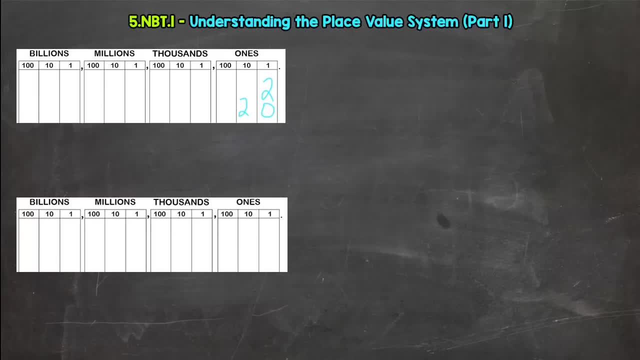 depending on which place they're in. So I'm going to come over here to the right to talk a little bit more about this. So let's start with our 2 again And our 20. And let's push the 2 over one more spot. 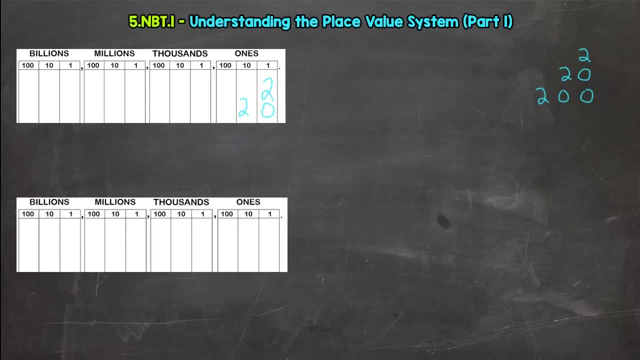 to the left and make its value 200.. Every time we push a number to the left one spot, our value increases by 10.. So think about it: If we have a 2 that's worth 2 and then a 2 that's worth 20,. 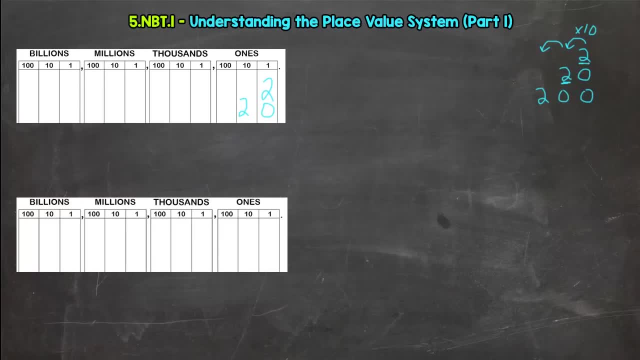 that 2 here is 10 times the value of this 2. And if we move it again, our value increases by 10. 2000.. Push it to the left again. Value increases by 10. By 10.. Okay, every jump to the left. 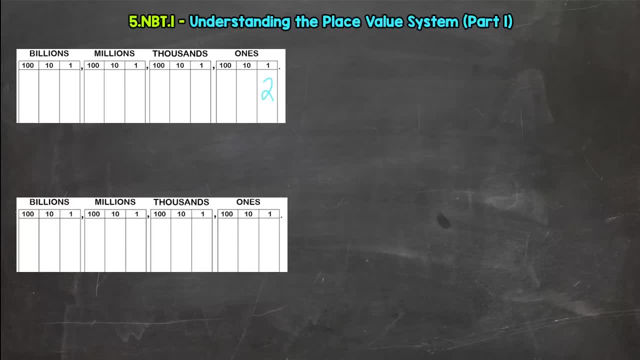 it's worth 2.. Its value is 2.. How about if we push it one place to the left, to the 10's place? Now we have a 20.. So we're going to talk about what happens to the value of numbers. 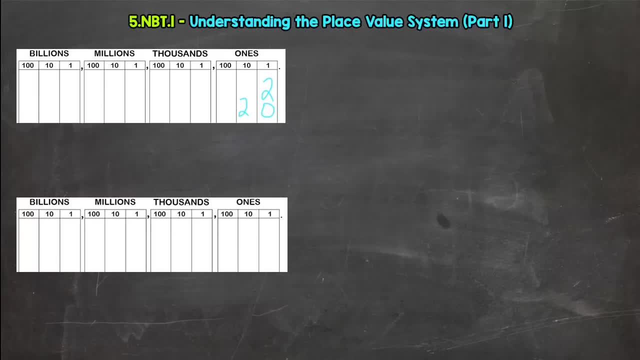 depending on which place they're in. So I'm going to come over here to the right to talk a little bit more about this. So let's start with our 2 again And our 20. And let's push the 2 over one more spot. 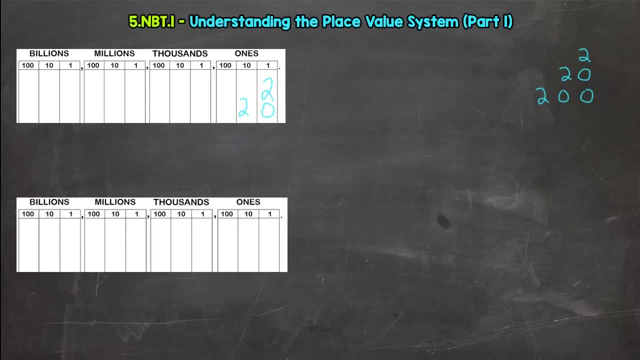 to the left and make its value 200.. Every time we push a number to the left one spot, our value increases by 10.. So think about it: If we have a 2 that's worth 2 and then a 2 that's worth 20,. 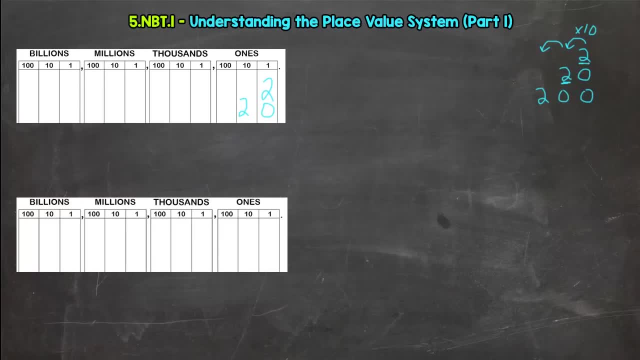 that 2 here is 10 times the value of this 2. And if we move it again, our value increases by 10. 2000.. Push it to the left again. Value increases by 10. By 10.. Okay, every jump to the left. 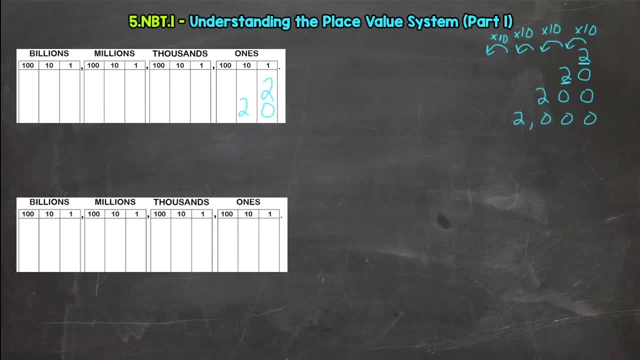 the value of that digit will increase by 10.. Okay, I'm going to write out a number here. We'll use 5's 55,555. we'll use as an example This 5 right here, value is 5.. If we take a look at the place, 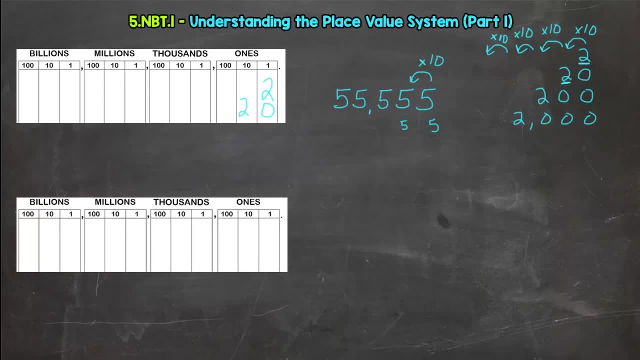 to the left. our value increases by 10.. This 5 would be worth 50.. Let's increase the value by 10 again, And we have 500.. Increase the value by 10 again. We have 5,000.. And then, if we increase the value by 10 again, 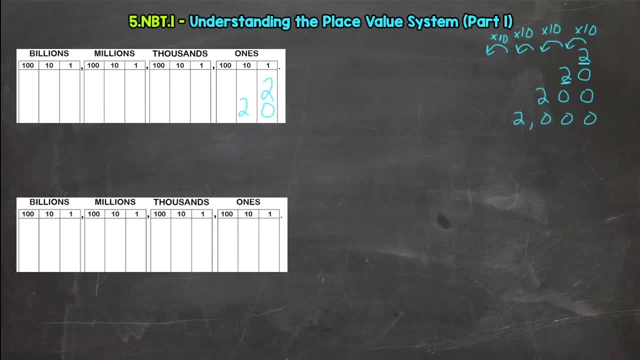 the value of that digit will increase by 10.. Okay, I'm going to write out a number here. We'll use 5's 55,555. we'll use as an example This 5 right here, value is 5.. If we take a look at the place, 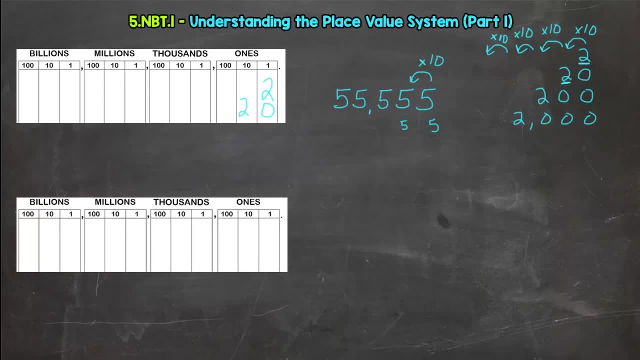 to the left. our value increases by 10.. This 5 would be worth 50.. Let's increase the value by 10 again, And we have 500.. Increase the value by 10 again. We have 5,000.. And then, if we increase the value by 10 again, 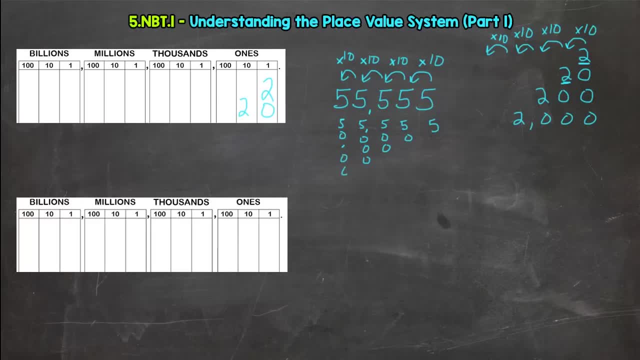 we have 50,000.. That looks like a decimal. That's a comma, That's a comma. Okay. So every jump to the left, the value increases by 10.. Now I'm going to do one more example here. How about we have a 7, and let's compare it to the value of the 7 in 700.. Now here we made two jumps. 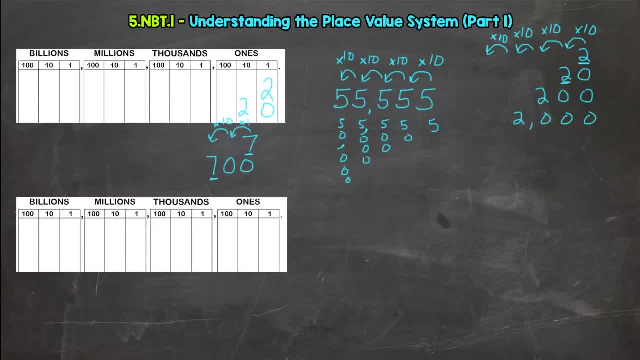 at once, which is 10 times 10.. So the value of this 7 here would be 100 times greater than this 7, because it's two spots to the left. Now we'll do some follow-up questions in Part 2 where we will apply this, so it will make a little more sense. 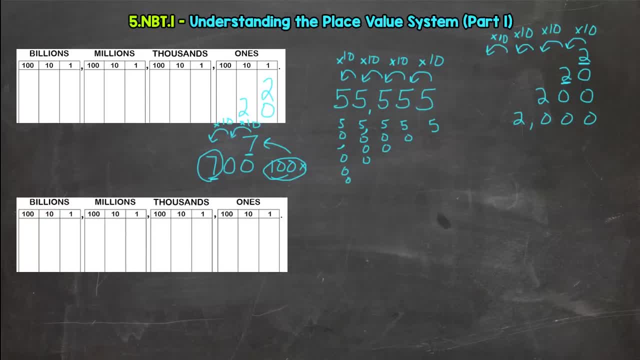 when we get into some 5th grade-type questions that have to do with the relationship here in our place value system. Now, if we go the other way, let's say we have an 80 here and we're comparing it to this 8. And we make a jump at this 8.. Well, we're going to change this relationships to 800.. So you want to do that because it's a really simple mechanisms. But here, if you go to the separate options, you start to remember that the equation is the answer. for Instruments, There's a common house value's number where two areas come together. and then you can start to multiply by 8.. When you say the difference between, theiffer means that it's equal to zero, and we're comparing it to this 8, and we make a jump by 10, that it is equal to 2380. 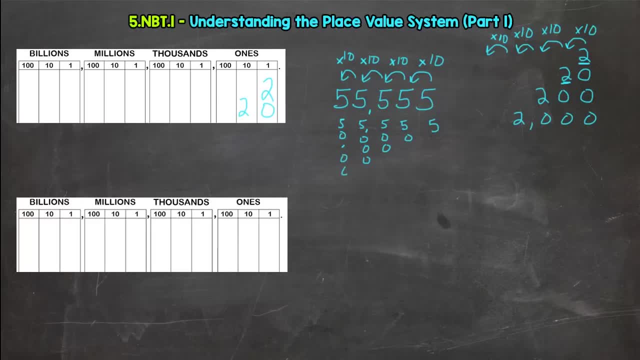 we have 50,000.. That looks like a decimal. That's a comma, That's a comma. Okay. So every jump to the left, the value increases by 10.. Now I'm going to do one more example here. How about we have a 7, and let's compare it to the value of the 7 in 700.. Now here we made two jumps. 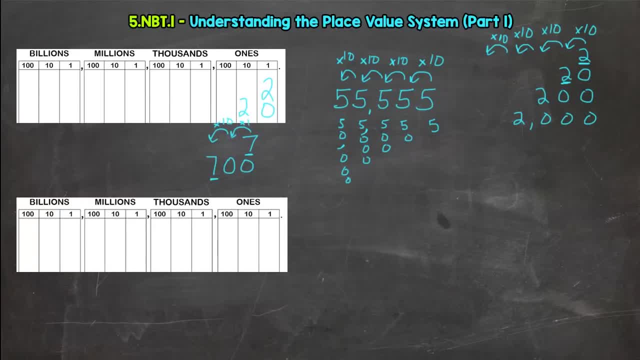 at once, which is 10 times 10.. So the value of this 7 here would be 100 times greater than this 7, because it's two spots to the left. Now we'll do some follow-up questions in part two where we will apply this. so it will make. 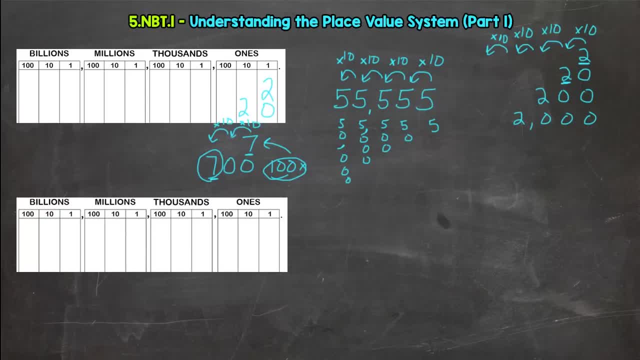 a little more sense when we get into some fifth-grade type questions that have to do with the relationship here in our place-value system. Now, if we go the other way, let's say we have a—an 80 here and we're comparing it to this 8.. 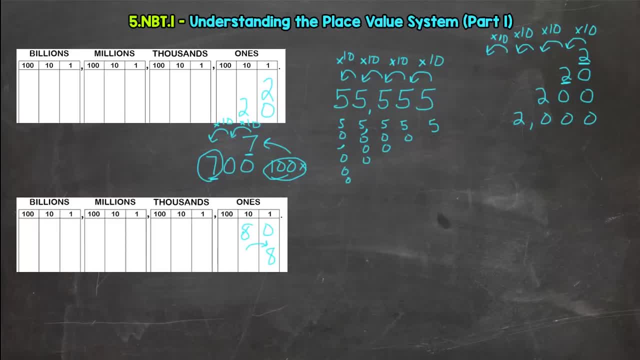 we make a jump to the right. every time we make a jump to the right or decrease the value by one place, we are taking 1 tenth of the value. so remember- I'll put a little note here- if we increase the value, which is a jump to the left, we 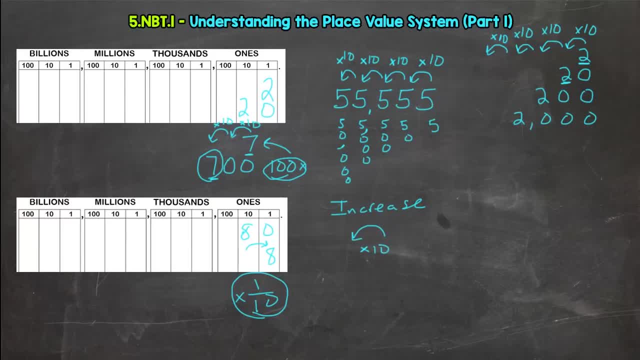 increase the value by 10, 10 times the value. if we decrease the value or make a jump to the right, we take 1, 10th of the value. so that same example will do 55,000, 555 every jump to the right. that 5 decreases in value by 1 tenth.